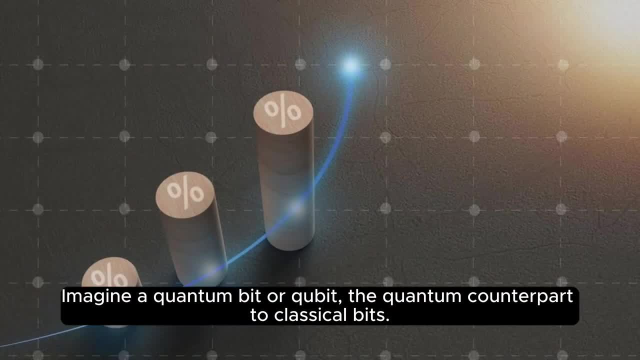 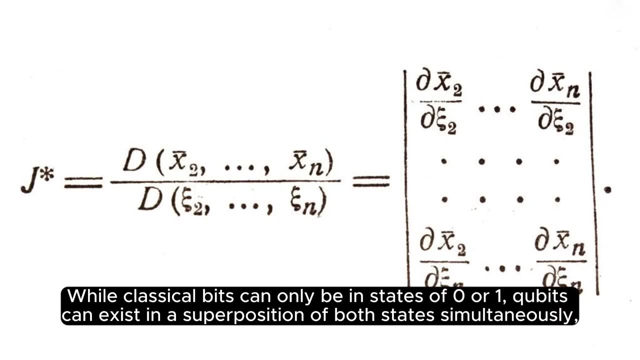 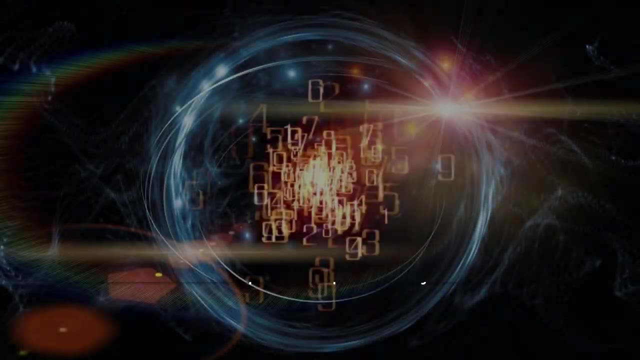 exist in multiple states at once. Imagine a quantum bit or qubit, the quantum counterpart to classical bits. While classical bits can only be in states of zero or one, qubits can exist in a superposition of both states, simultaneously expanding the potential computational power of quantum computers exponentially. 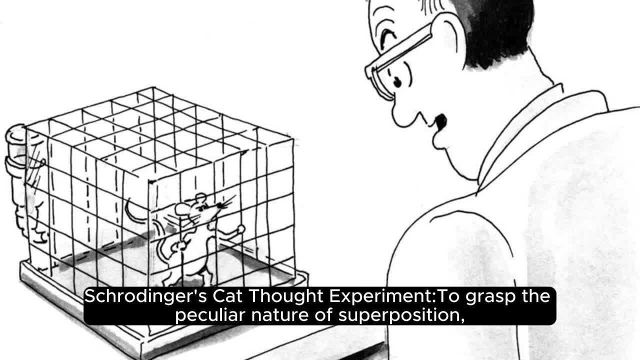 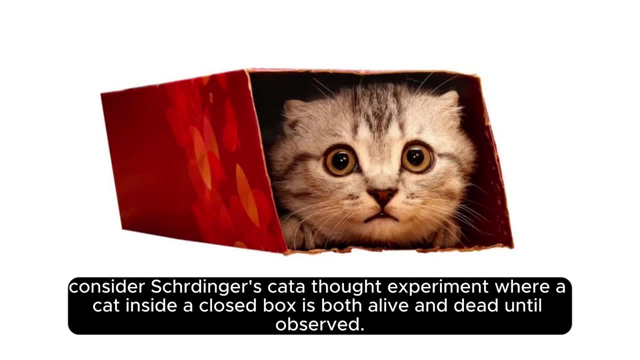 Schrödinger's cat thought experiment. to grasp the peculiar nature of superposition, Consider Schrödinger's kata thought experiment, where a cat inside a closed box is a cat inside a closed box is both alive and dead until observed. This illustrates the concept. 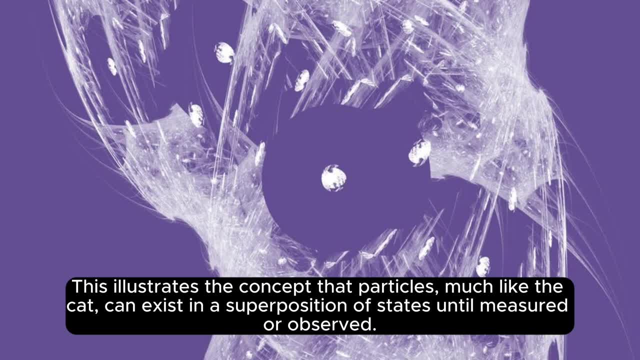 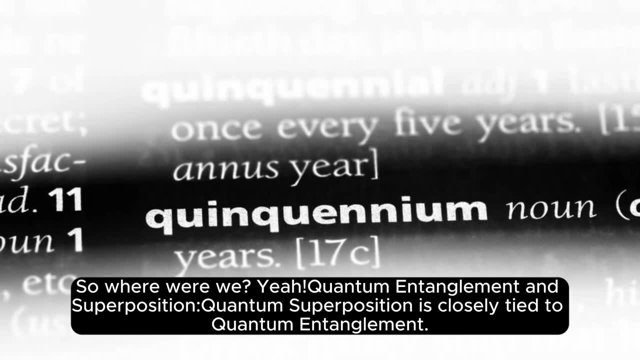 that particles much like the cat can exist in a superposition of states until measured or observed. Next episode will be on this topic. So where were we? Yeah, quantum entanglement and superposition. Quantum superposition is closely tied to quantum entanglement. 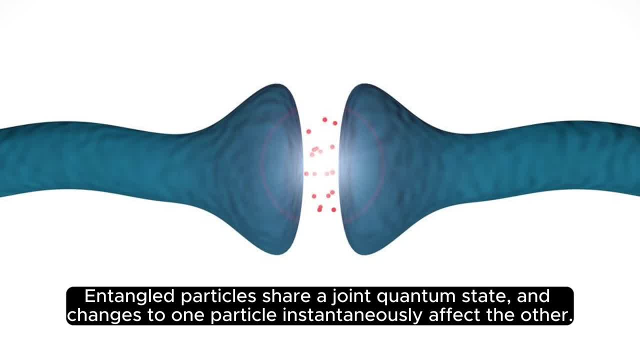 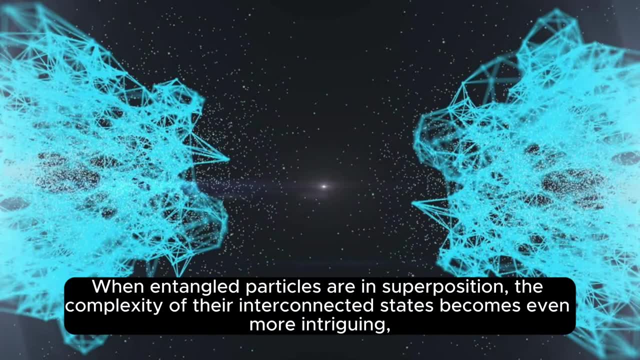 Entangled particles share a joint quantum state and changes to one particle instantaneously affect the other. When entangled particles are in superposition, the complexity of their interconnected states becomes even more intriguing, Showcasing the richness and intricacies of 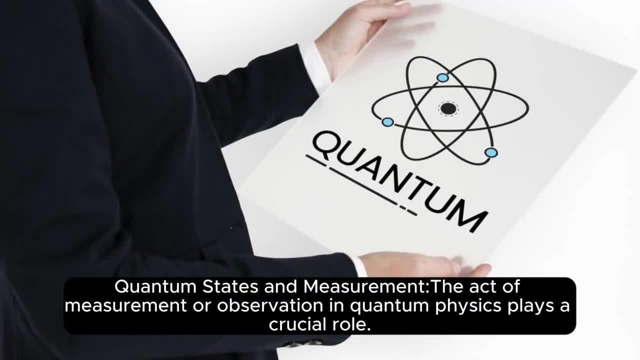 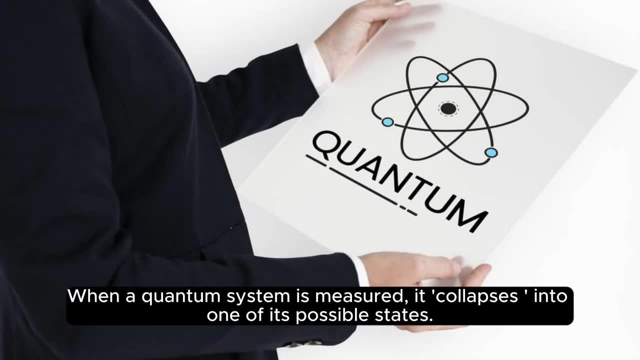 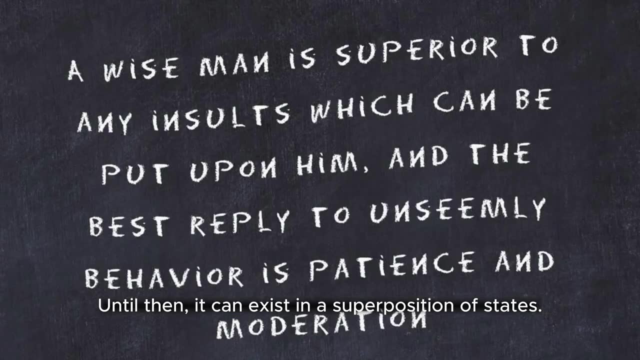 the quantum world, Quantum states and measurement. the act of measurement or observation in quantum physics plays a crucial role. When a quantum system is measured, it collapses into one of its possible states. Until then, it can exist in a superposition of states. This is 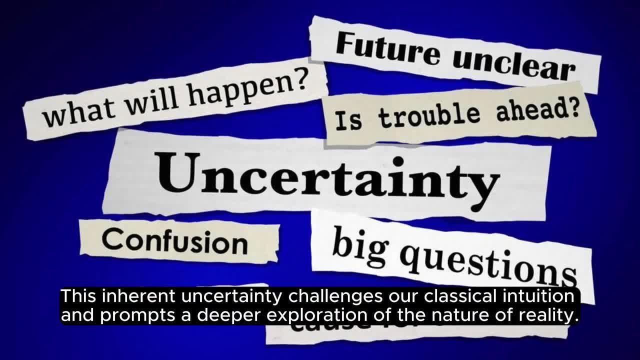 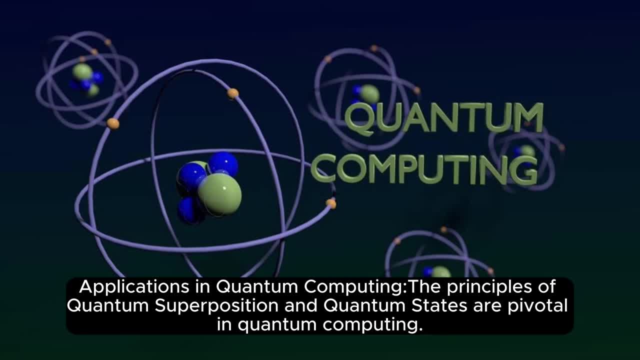 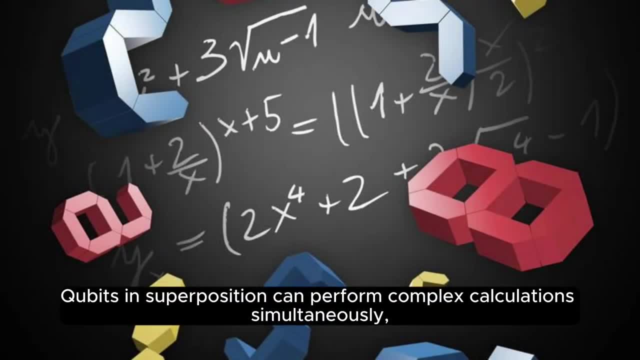 the first time that a quantum system can exist in a superposition of states. This inherent uncertainty challenges our classical intuition and prompts a deeper exploration of the nature of reality. Applications in quantum computing that principles of quantum superposition and quantum states are pivotal in quantum computing. Qubits in superposition can perform. 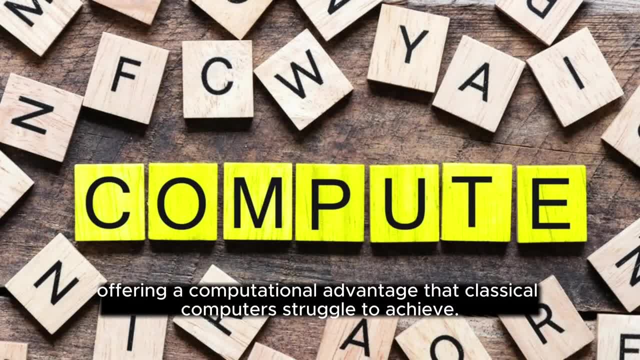 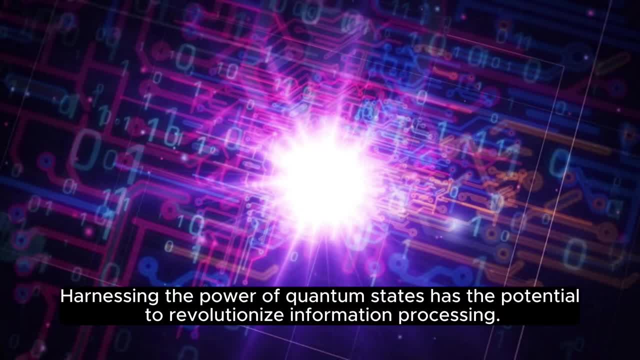 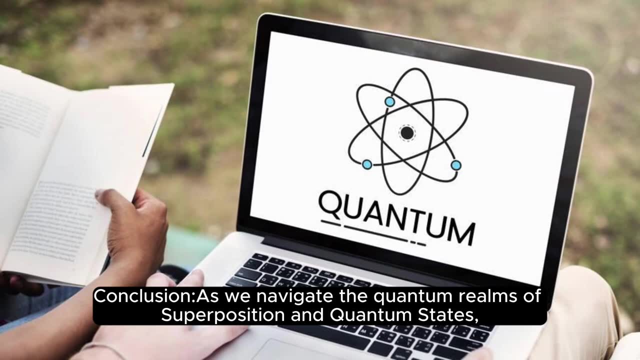 complex calculations, simultaneously Offering a computational advantage that classical computers struggle to achieve. Harnessing the power of quantum states has led to the evolution of quantum reality and has the potential to revolutionize information processing. Conclusion: Sway, navigate the quantum realms of superposition and quantum states. We encounter a reality.